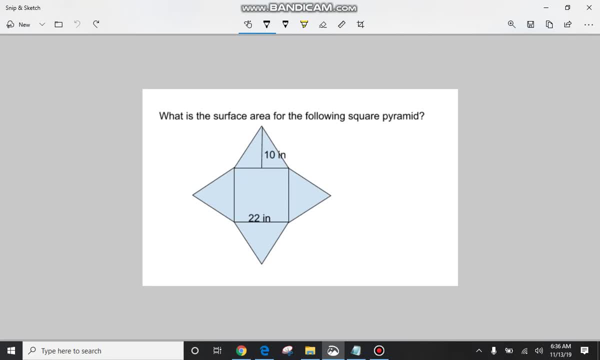 Okay, all right. Now let's find the surface area. So there are five sides to this figure. You get the square And let's find the area for that. So I'm going to do a little error over here. The area for this: we know it's a square, So we know that this is 22.. Then we know that the area is going to be 22 times 22. And that's going to be the area. So two times two is four. Two times two is four: Zero. 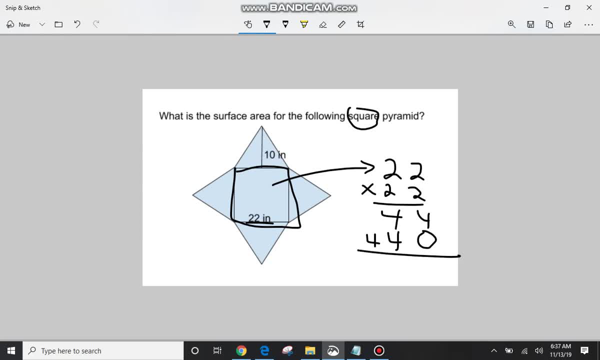 Four, Four, And I'm going to add them And I get four, eight and four, So the square is 484 square inches. Now I'm going to do the triangle, Do a little error here. This is one half Base. All right, the base here is 22 due to this side here, So 22.. And then the height, which is 10.. 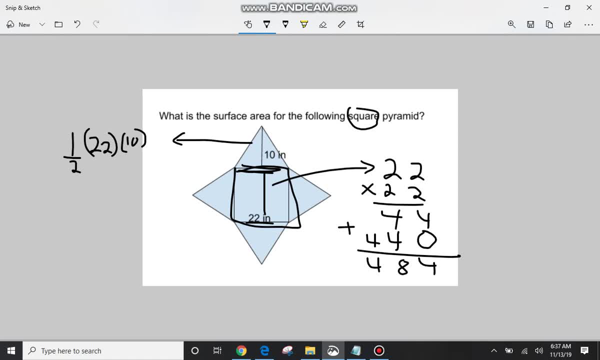 Now I love 10.. I'm not going to take half of 10.. I'm going to take half of 22.. So half of 22 is 11.. 11 times 10 is 110.. Now there are two triangles here. This, or actually there's four: One, two, three, four, And they're all the same, And that's going to be standard for any square pyramid. They're going to flap up and all be the same. So I'm going to multiply this guy by four. 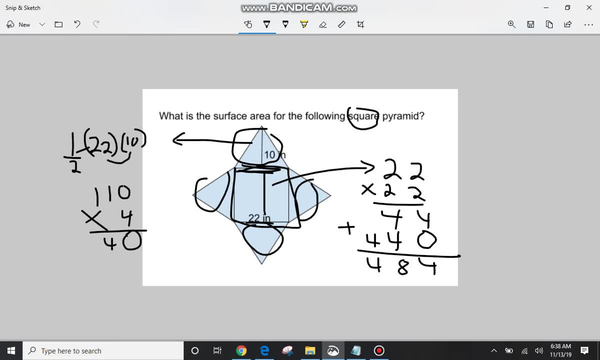 Because there's four triangles: Zero Four, Four. All right, now I'm going to add these two together, Because this is my square And these are my four triangles, So I'm going to go over here to a little cleaner spot. 440. Plus 484. 412. 924.. 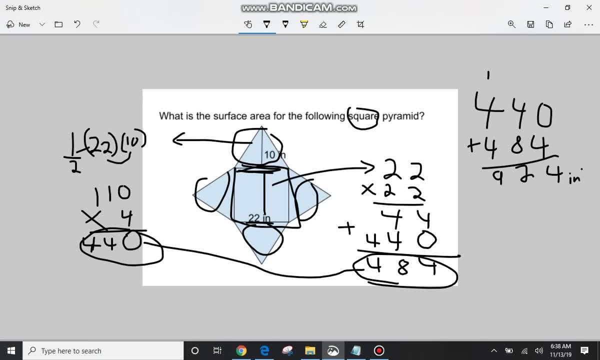 Four inches Square And there's the area for that square pyramid.